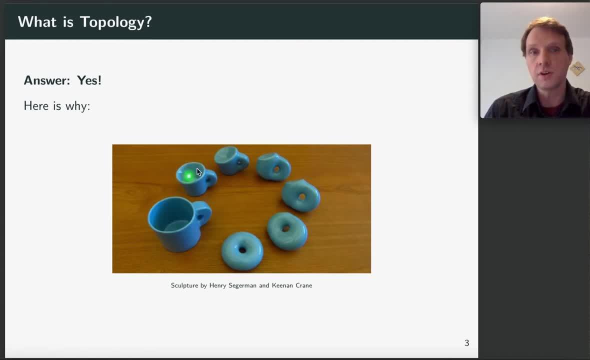 And you see what you have to do. You have to raise the bottom of the coffee cup and thicken the handle until you end up with this donut shape shown here, And mathematicians like to call this shape the torus. So here's a way to go from the coffee cup to the donut shape. 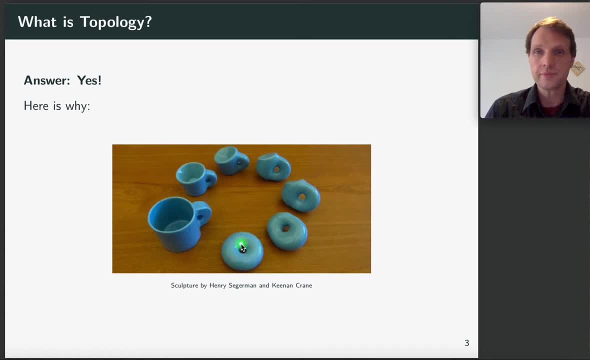 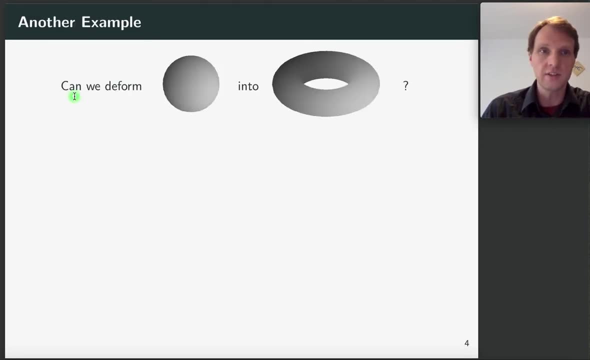 From the top of the coffee cup all the way to the torus. So the answer to this question was yes. There's another question that we can consider. So it looks like this: Can we deform the surface of the sphere into the surface of the donut? 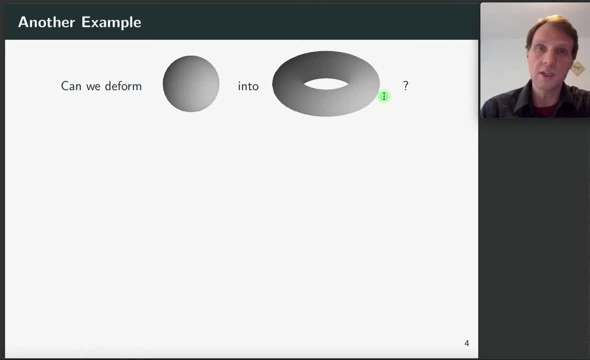 And you can try this, And the answer seems to be no. in this case, The question is: how do you actually see this right? How do you prove that something cannot be done? And mathematicians are usually like this: They're usually not happy with the answer. 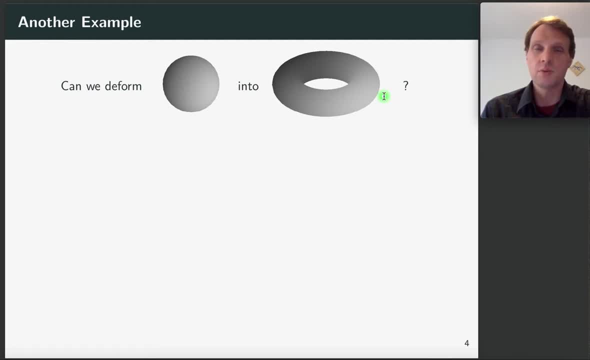 I just tried a few times and it didn't work. They want to know the precise reason. They want to have a watertight argument why something cannot be done, And in this case, this is where algebraic topology comes into play, And if you want to know the explicit answer to this question here: 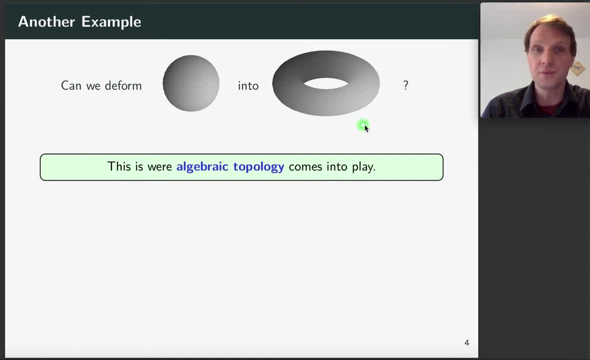 I'll invite you to attend the course at Cardiff where we discuss this. What I want to do in this brief overview is I want to discuss a slightly easier question, which looks like a Minecraft version of this question shown here. And here's the question. 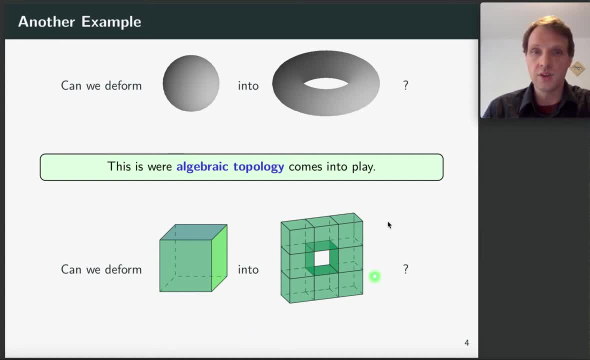 Can we deform this cube into this Minecraft version of the donut shown here? So what makes this question easier than this one here? Well, here, these shapes are made out of vertices, edges and faces, And that's something that we can count right. 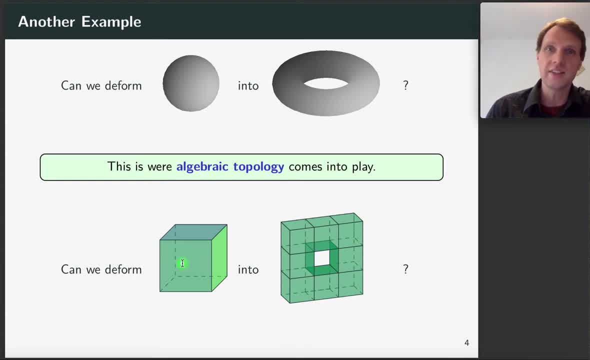 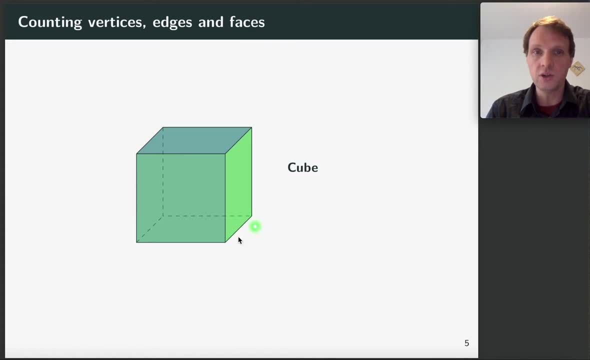 So that brings us back to numbers. So let's do that, Let's count the number of vertices, edges and faces. Here's the cube again. And the cube has eight vertices, So four at the bottom and four at the top. 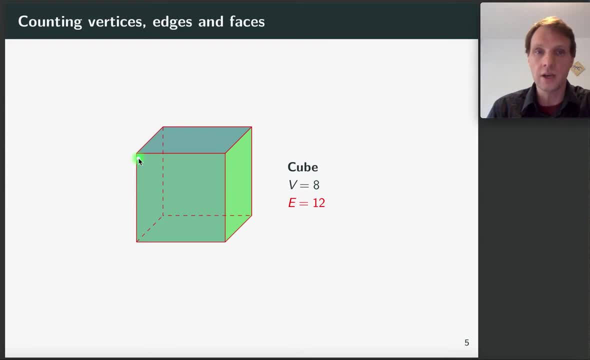 And it also has twelve edges shown in red here. So you have four that make up the top, four that make up the bottom and four in the middle. Twelve edges, And since this is also the six-sided die, it also has six faces shown in red here. 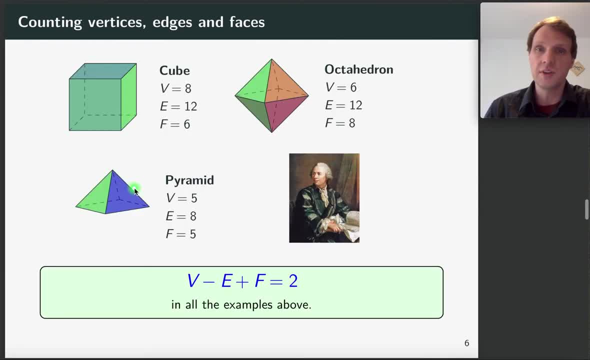 You can compute these numbers for all kinds of different shapes, and this is done on the next slide. So here you have the numbers for the octahedron, which looks like this, and for the pyramid, which looks like this, And the Swiss mathematician Leonhard Euler. 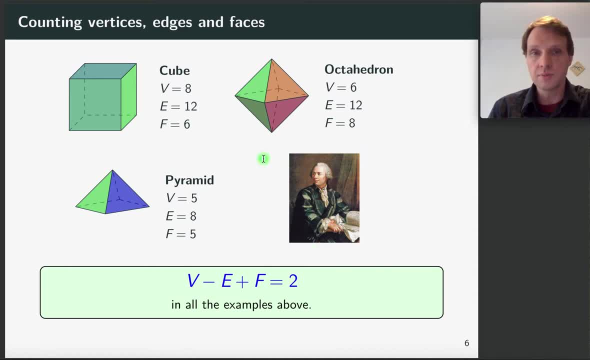 who lived in the 1700s, made a curious observation about these numbers, namely that if you take the number of vertices, subtract the number of edges and add the number of faces, then in all of these examples you get the number two. 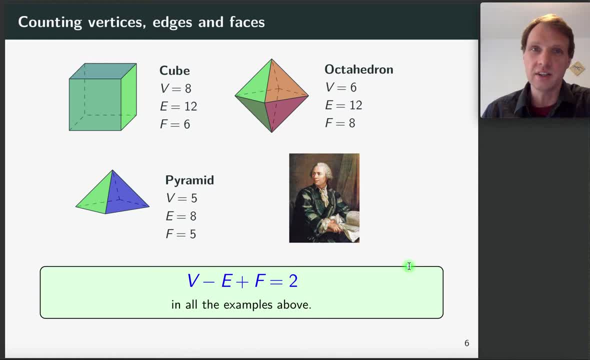 And you can pause the video here and check that my computations are correct and that you indeed always get the same number. There's another curious thing about this number- vertices minus edges plus faces- and that is that it doesn't change if I deform my shape. 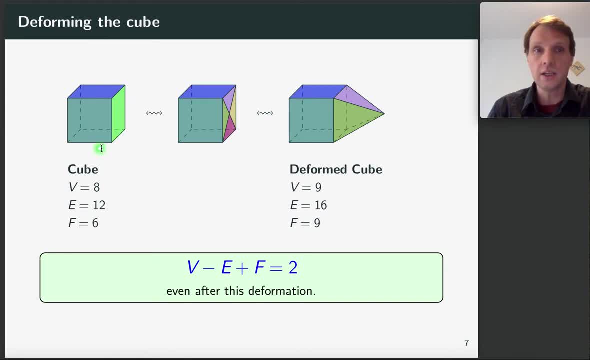 So here's what I mean by that. Let's take the cube again. let's take this bright green face of the cube, and one thing that we can do to deform the cube is we can just add another vertex in the middle, which creates also these new edges. 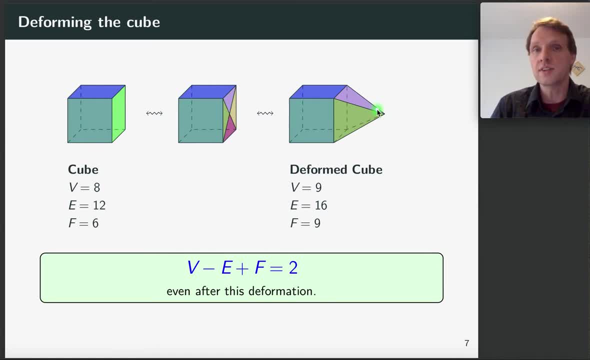 and these triangles here, And then we can move this vertex anywhere we like, so, for example, to here, And that deforms the cube into a new shape. How does that change the numbers, though? So let's look at the number of vertices. 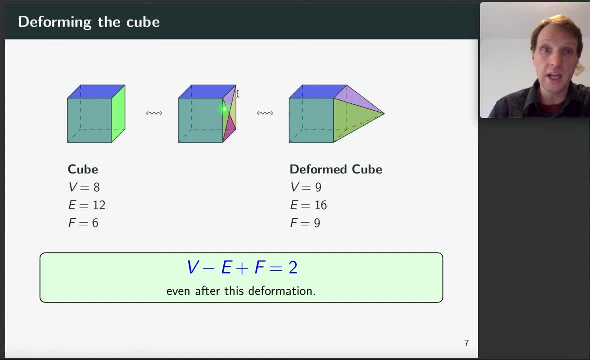 Here we had eight vertices, and we added another vertex in the middle, so now we are at nine. What about the edges? Here we have 12 edges, and we added these four edges here, and so we now add 16.. What about the faces? 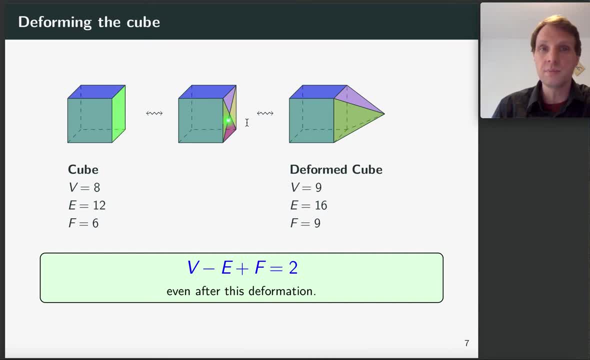 We removed this bright green face here and replaced it by these four triangles that you can see in this picture here. So we removed one and added four, which brings us from six up to nine, And now you can check again that if you take the number of vertices. 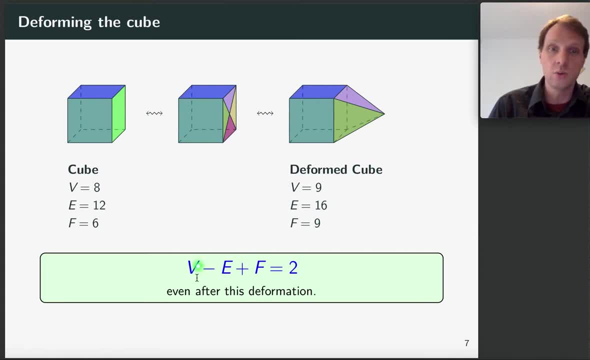 minus the number of edges, plus the number of faces, you can get two. And the most surprising thing about this number of vertices minus edges, plus faces, is that it also doesn't change under any other deformation that you can think of, So no deformation that you can perform on the cube. 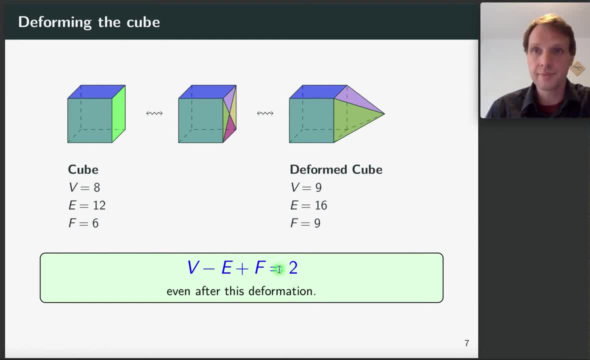 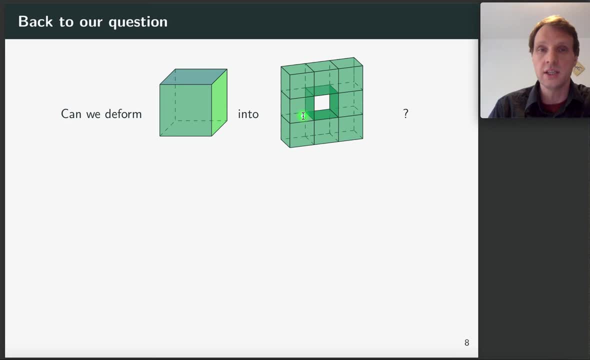 will change this number. And that brings us back to our original question: Can we deform this cube into this donut here? Because how we can approach this question is we can just compute the numbers for both of them And if we can deform the cube into the donut, 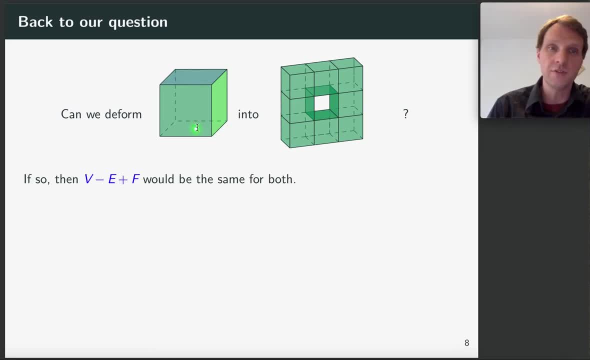 then the numbers are equal, right? If we can deform one into the other, the numbers will be the same. So let's do that, Let's compute these numbers. So for the cube, we've already done that, and the number turns out to be two. 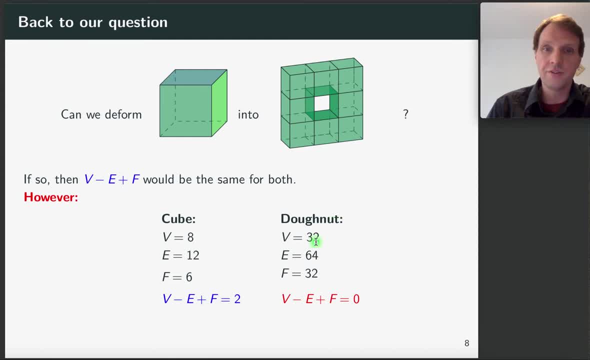 as shown here, For the donut you have 32 vertices, 64 edges and 32 faces. So if you compute this number here, then vertices minus edges plus faces turns out to be zero. And then you count this again. 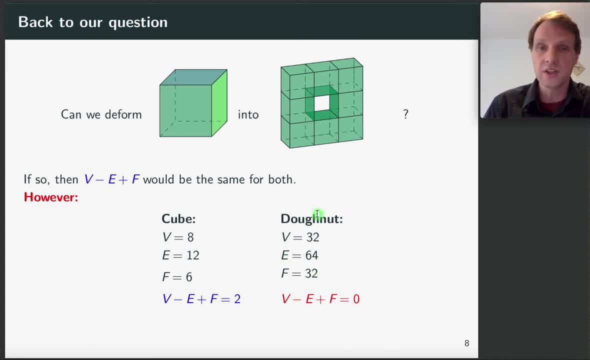 because that's a lot of vertices, edges and faces to count. But no matter what you do, you always will end up with zero, And there's actually a reason for that, And the reason is that this surface has this hole in the middle. 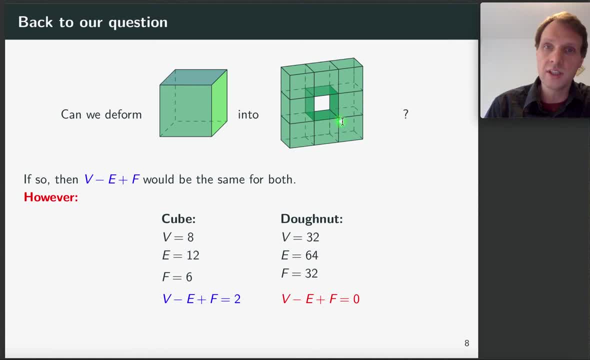 So this number allows us to detect this hole, And that's the reason why this number goes down, And it also helps us to answer this question now. This is now a watertight argument that the cube cannot be deformed into this donut. 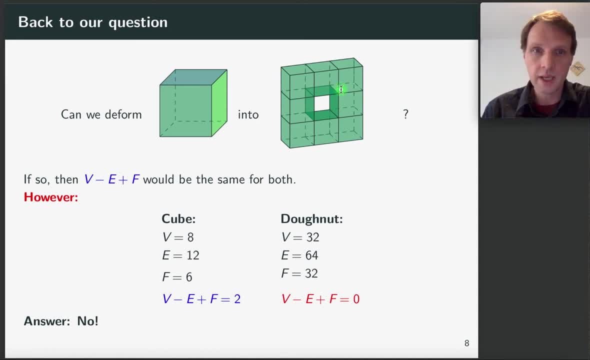 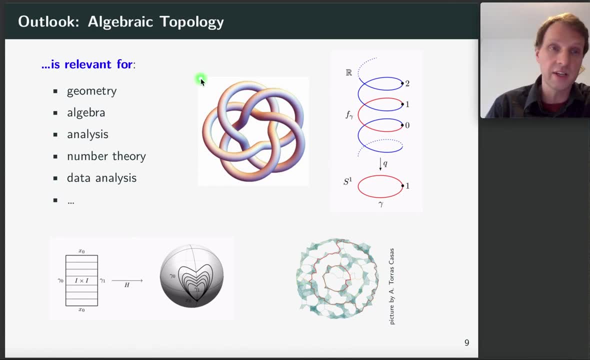 So the answer is no, And considerations like this come up in a lot of other different, in a lot of other areas of mathematics. So- and here I just listed some of them where this plays a role, And I want to highlight a few of them- 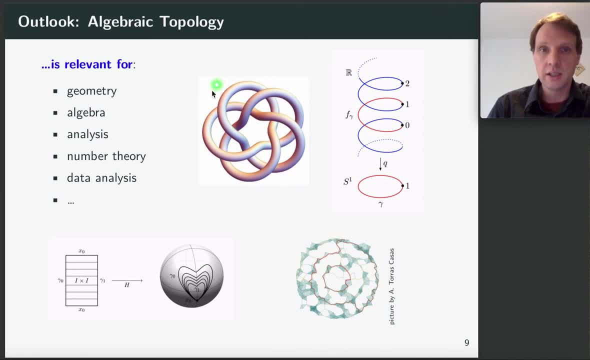 So, for example, whenever you need something in an area of mathematics that has to deal with knots or being knotted, then you end up with something that is related to topology or algebraic topology. And another good thing about numbers like the one that I've presented on these slides: 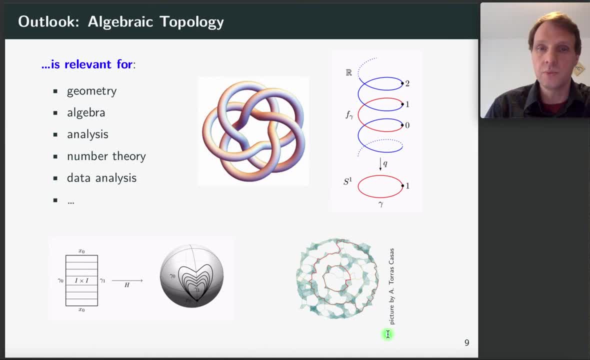 is that they can be calculated using a computer And they tell you something about the number of holes in your data, the number of data sets. They also tell you something about connected components of your data set, And I had a PhD student working on this.